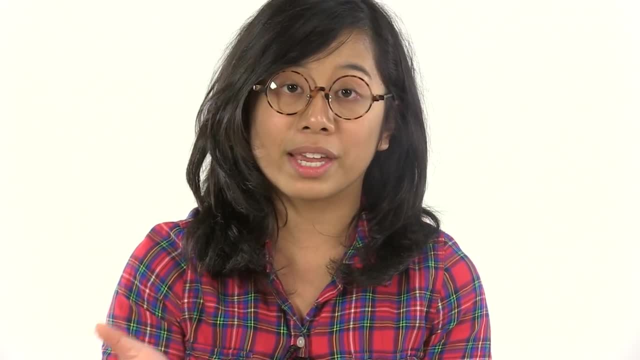 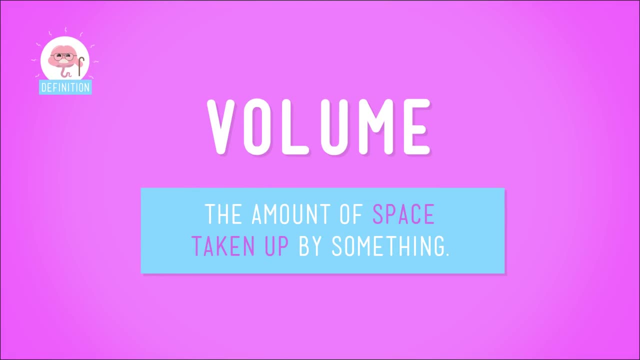 doctor's office, the first thing they do is have you stand on the scale so they can measure how much you weigh. As for taking up space, another way of thinking about it is that all matter has volume. It simply fills the area it's in. When you pour water into a glass, for example, the 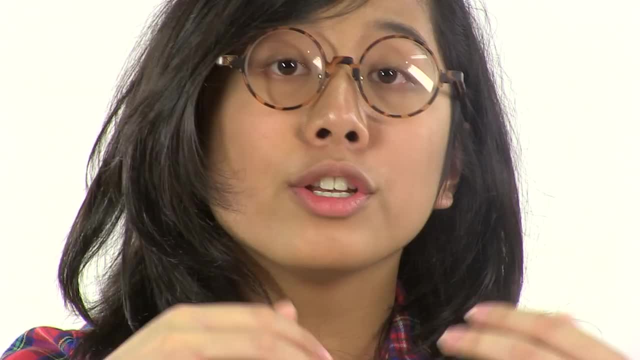 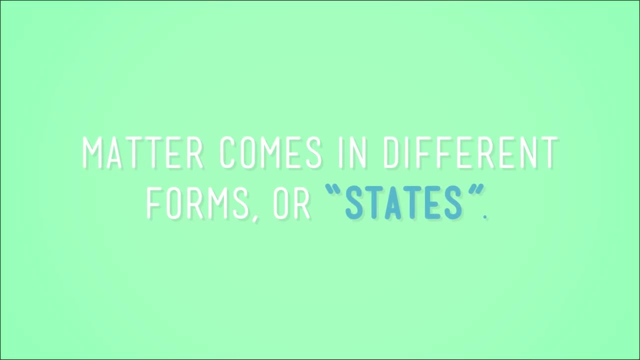 water's volume is the amount of space that it takes up in the glass. So all matter has volume and weight. but it sure doesn't all look the same. Well, that's because matter comes in different forms or states. Liquids are a state of matter that I'm sure you're familiar with, If you've 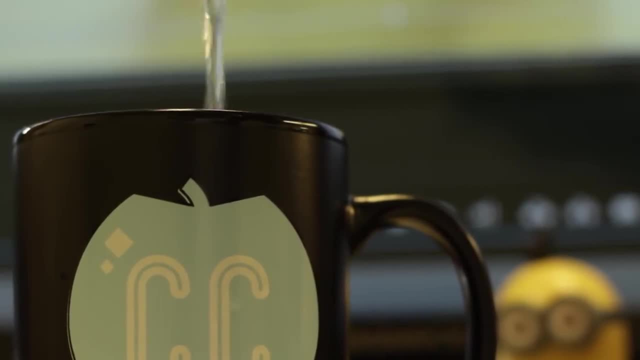 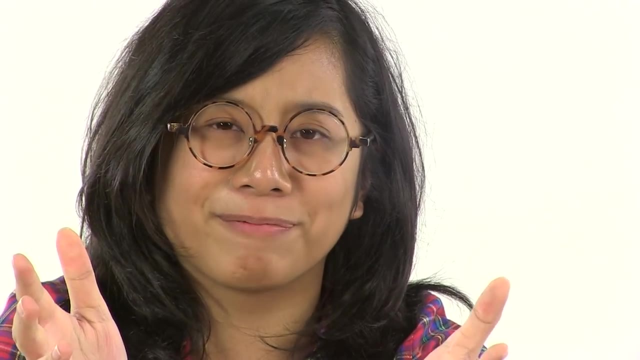 ever poured yourself a drink while trying to watch TV, you might have noticed that liquids take up space, because once the space inside your glass is full, gah right On the carpet. Sorry, Mom. You also know that water has weight if you carry a water bottle As you. 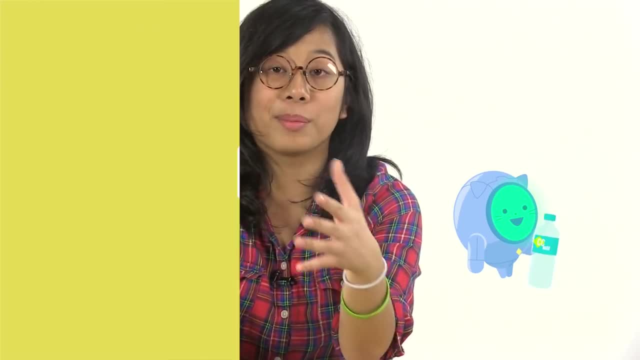 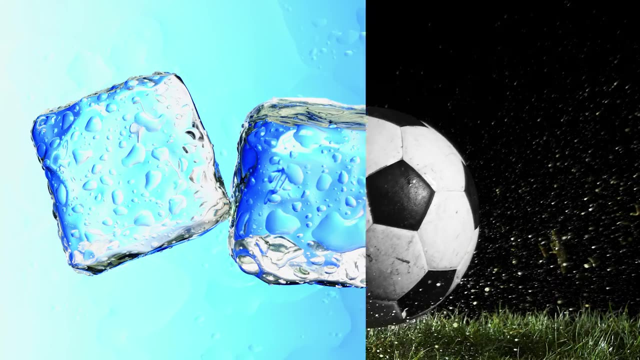 drink from it, it gets lighter because you're removing water from it. Solids are matter too, of course. probably the most obvious kind. Rocks are solid, and so is ice, which is just solid water. Soccer balls are solid, iPads, your pet Fluffy and every single guy in One Direction, And just 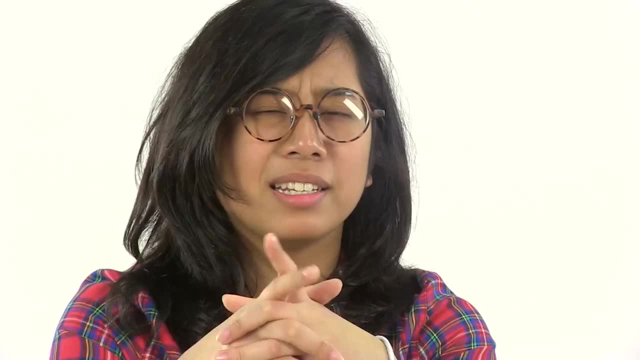 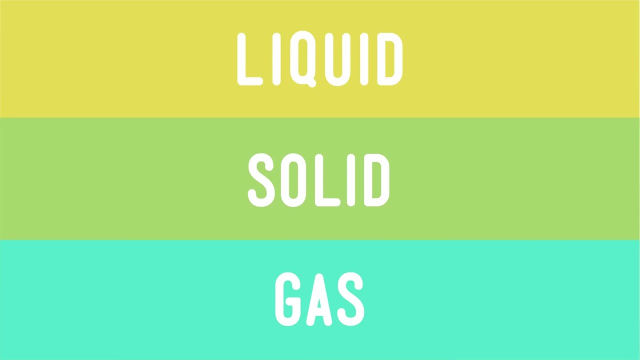 like rocks. all those things have weight and take up space. Now you know what's weird. Sometimes matter can't be seen or felt, but it's there Like the air we breathe. Air is an example of gas, the third main state of matter, And I probably 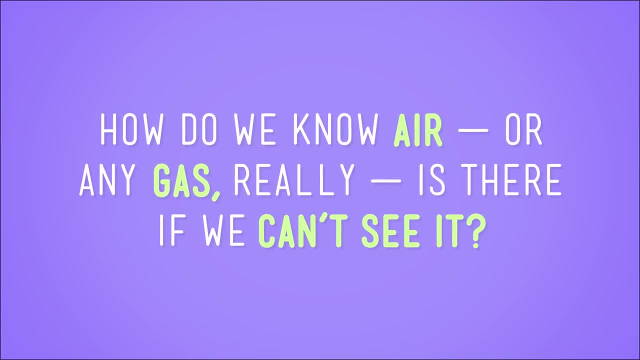 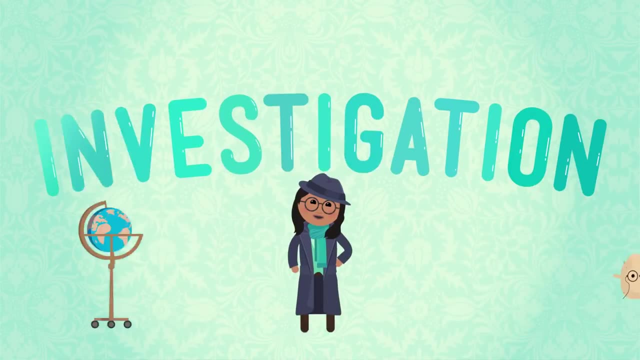 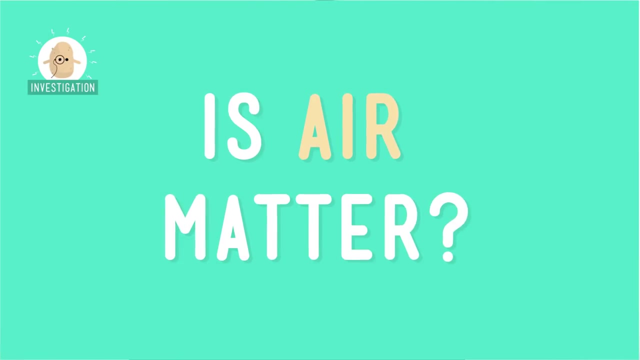 know what you're thinking. How do we know air or any gas really is there if we can't see it? Well, we can prove it by doing an experiment Science. Hmm, Let's start by asking the question: Is air matter? Because if it is, it should take. 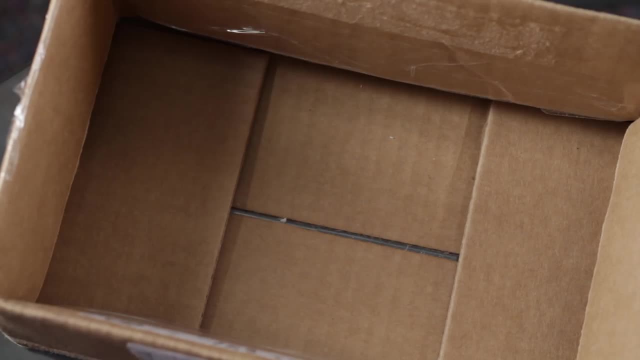 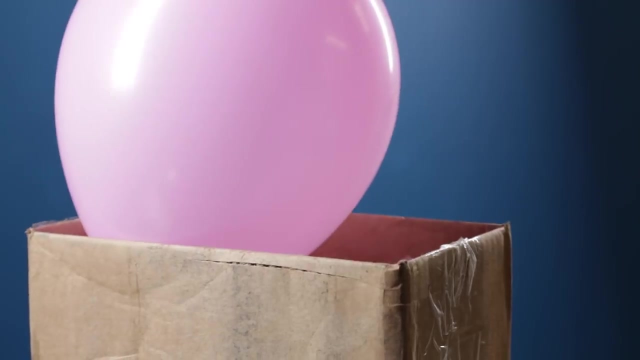 up space and have weight right To see if air takes up space. lookit, I can easily drop an empty balloon into this little box, But a full one won't fit. That's because the air that fills the really space inside the balloon is bigger than the space inside. 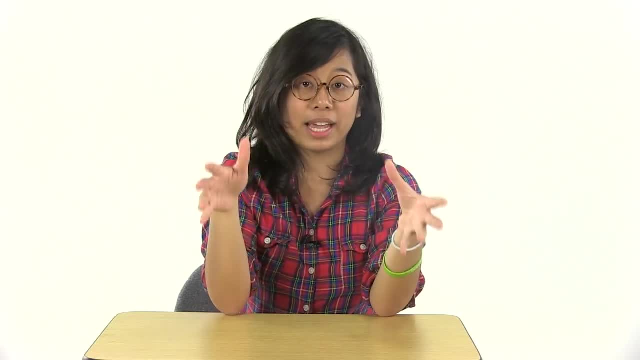 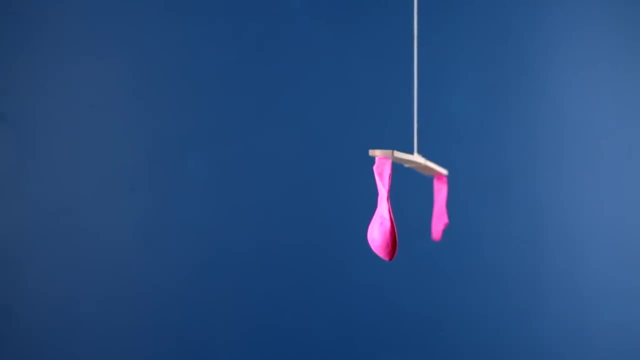 the box. Now does air have weight? Let's try something else. Take two empty balloons and tape them to the ends of a meter stick. Then we'll hang the meter stick on a string so that it's perfectly balanced. Now let's see what happens if we blow up just one of the balloons and put it back on.